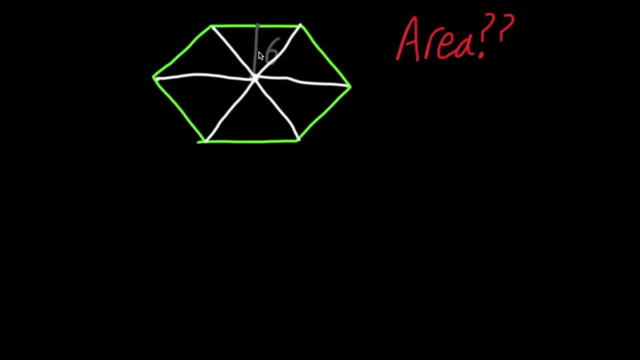 But how do we find the area of this triangle? Well, first of all, if we have 6 triangles and we have 360 degrees all the way around in the circle, if we divide that by 6, we get 60.. 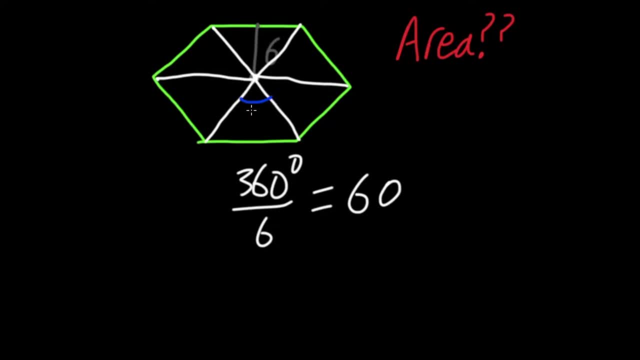 This means that each one of these triangles has this corner. This means that each one of these triangles has this corner length of 60 degrees, And if we went all the way around, we'd have 60,, 120,, 180,, 240,, 300, and 360. 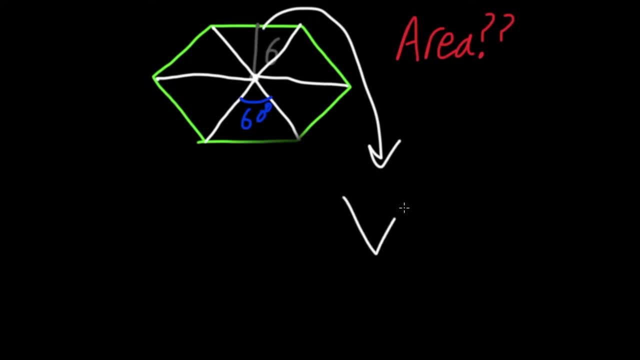 But if we look at this triangle here, we have split it up not just to this triangle but to two smaller triangles with this line here. That means that if we just take one of these triangles here, so say, this side, this is only 60 degrees. 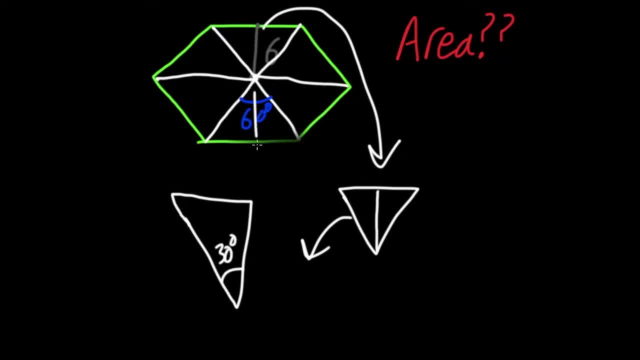 So we have 60 degrees. So we have only 30 degrees, because it would be half of the 60. And we have our 6 apart from here. So this side length here is 6.. That means we can find this side length here using trigonometry. 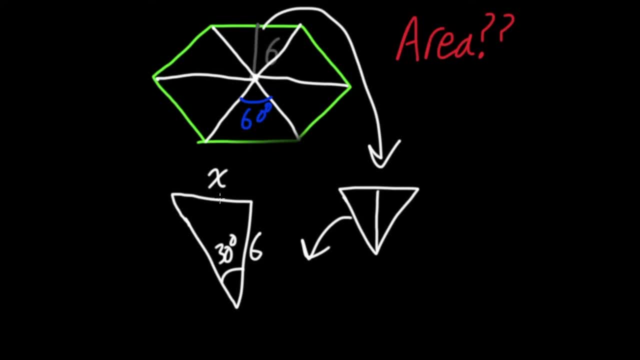 So let's just call this side length x, Because this is opposite over adjacent, we have: tan of 30 is equal to x over 6.. If we multiply both sides, we get 60.. If we multiply both sides by 6, we get x equals 6, tan 30. 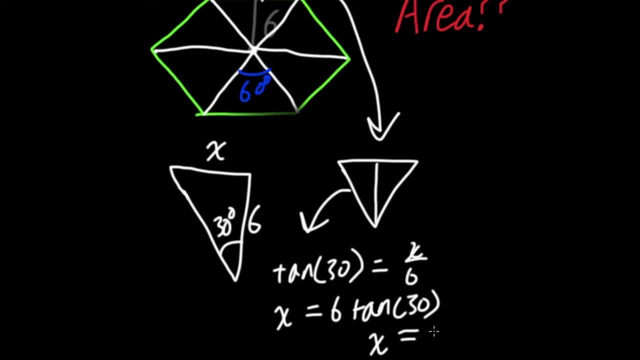 And if you type that into your calculator, you'll get x is equal to 3.5 rounded. Now remember this x here is only half of this triangle, So if we went all the way across, it would be double this. 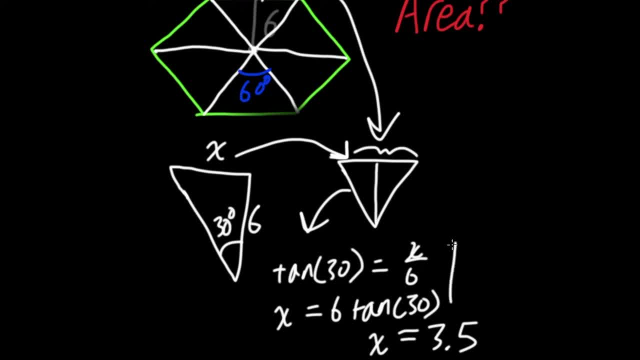 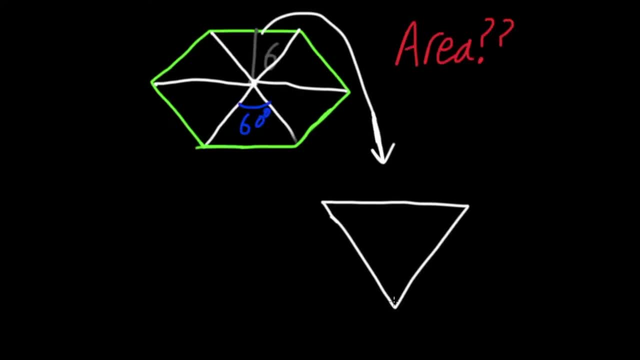 So this entire length is actually 3.5 times 2,, which is 7.. This means that now not only do we know the height of this triangle here is 6,, but we also know that the base is 7.. 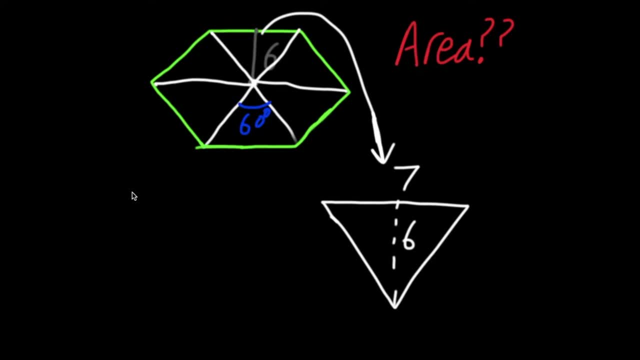 We can now use the formula to find the area of this triangle. The formula for the area of a triangle is 1 half base times height. So our area is equal to 1 half base, which is 7, times our height, which is 6..